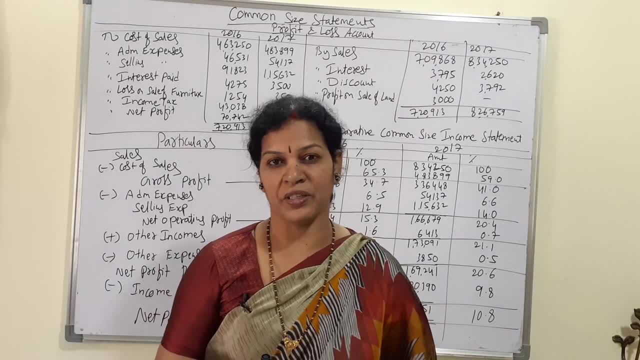 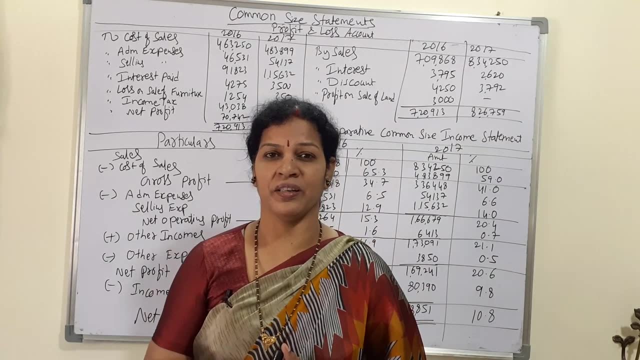 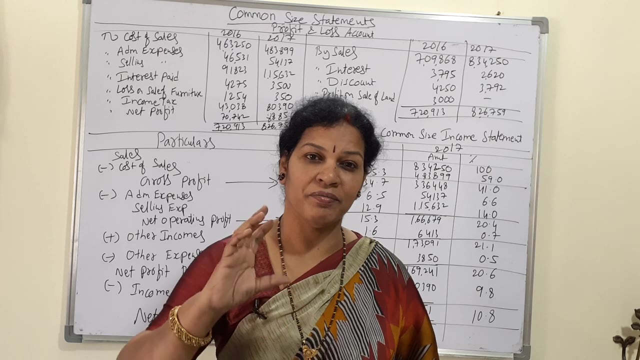 There is a small drawback in the comparative statements, Like we were comparing one year to another year. But what is the base we are not taking? That base is just simply last year to this year. We won't be knowing exactly the value and how much is increasing. and what is the base of that that we won't be knowing? 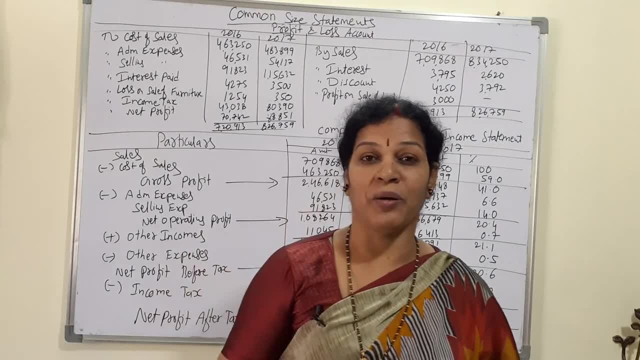 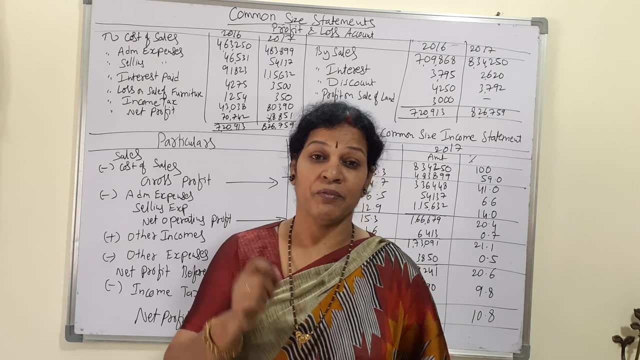 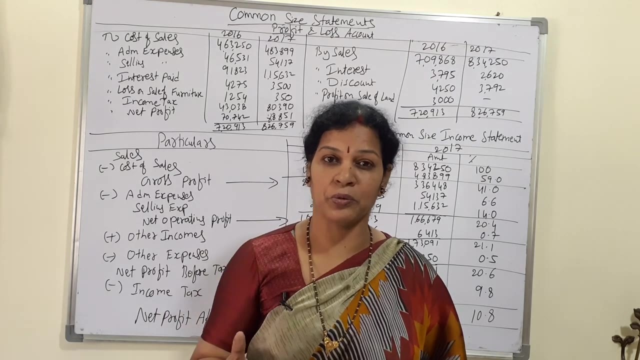 So, to overcome this problem, we will be going for the common size statement. In common size statements, what happens? We take only one particular amount as base, One particular transaction as base, and will be calculating and will be will be work out in total pro forma. 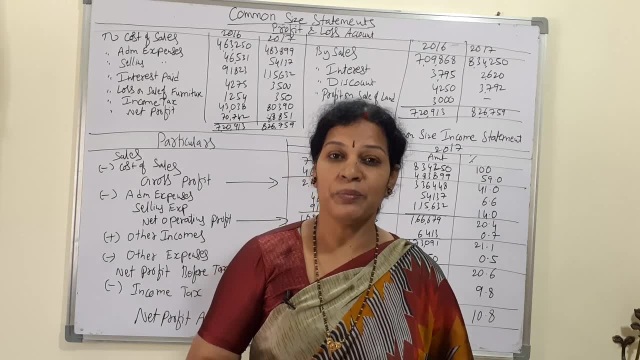 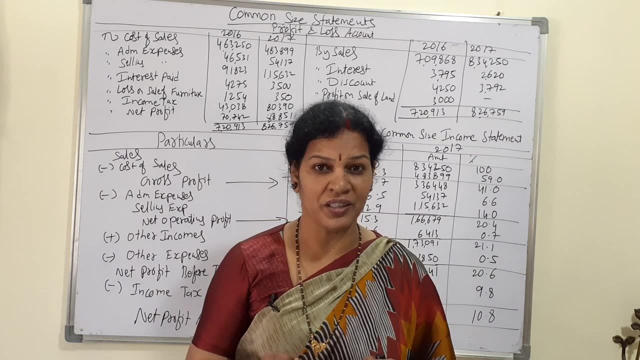 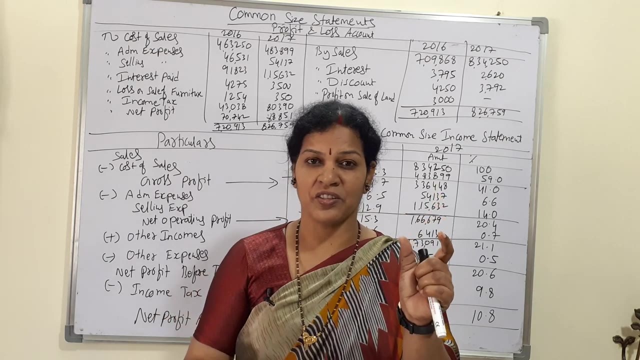 So what is that base? Suppose if you go for income statement, common size income statement, The base will be always sales. Are you getting it? The base will be always sales. Whatever sales we have with that base, all the transactions we are going to calculate as percentage. 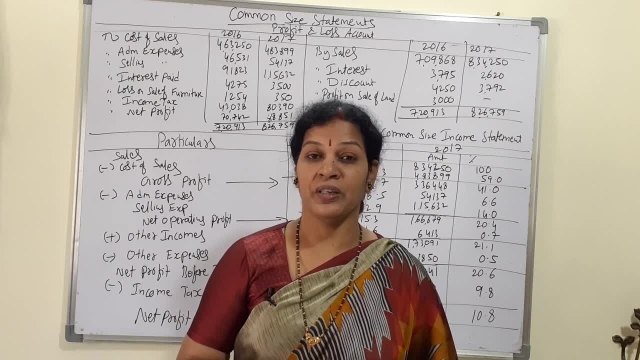 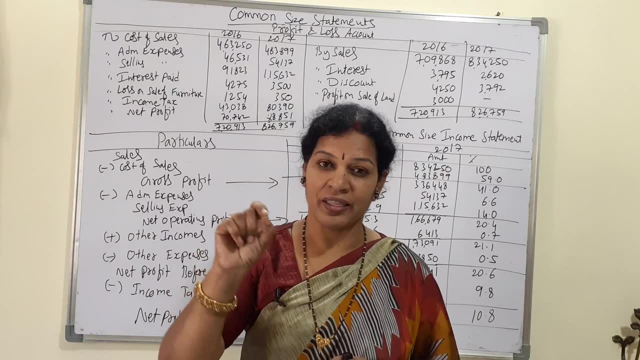 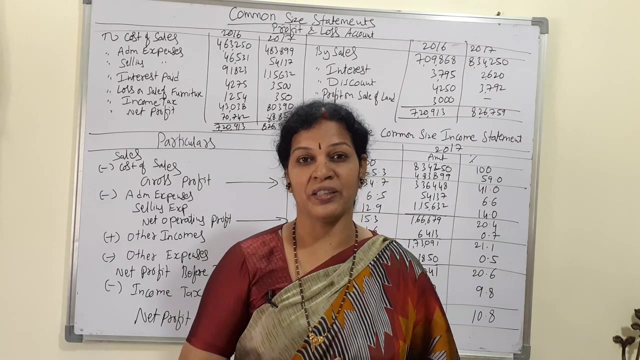 In the same way, if you go for balance sheet- Common size balance sheet- Here we will have the base as total assets or total liabilities, That amount as a base, Not the previous year amount. So in that way we are going to calculate this common size statements. 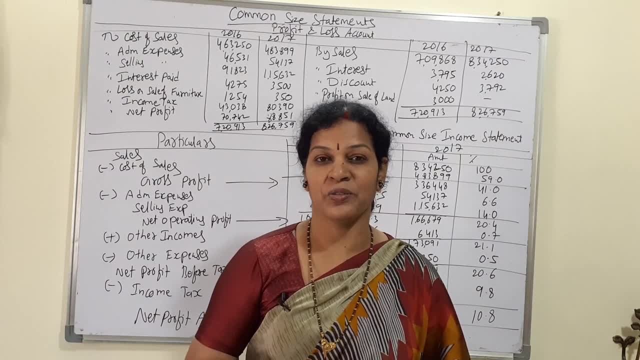 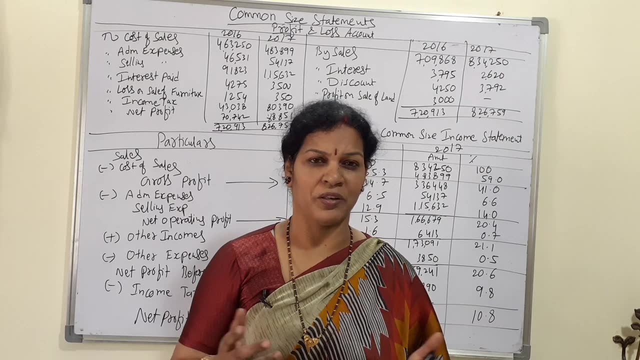 Don't worry. while work outing problems, you will have much idea, So nothing to worry. So today, in this episode we will see common size income statement. How we can calculate Pro forma is same, Just like comparative income statement. what we have done: Same pro forma. 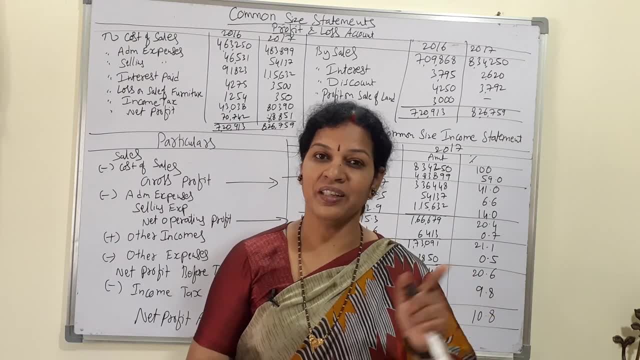 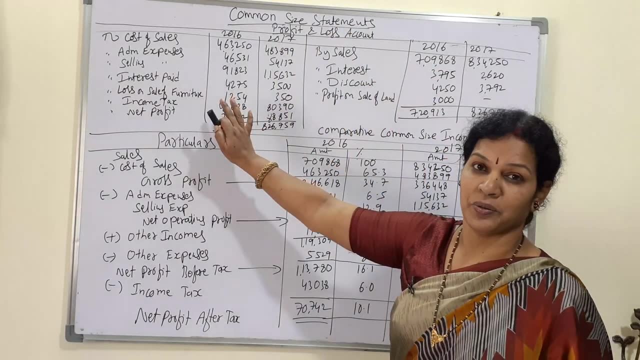 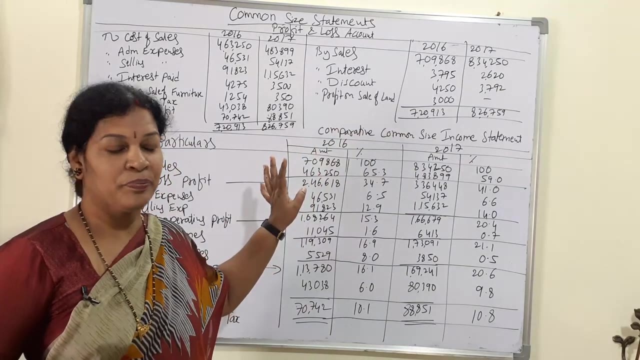 But common size we are taking rather than comparative. So here, common size statements we have. according, What is given to us is profit and loss account. Out of this we are going to prepare comparative common size income statement. Now for this, remember the pro forma: same as usual. 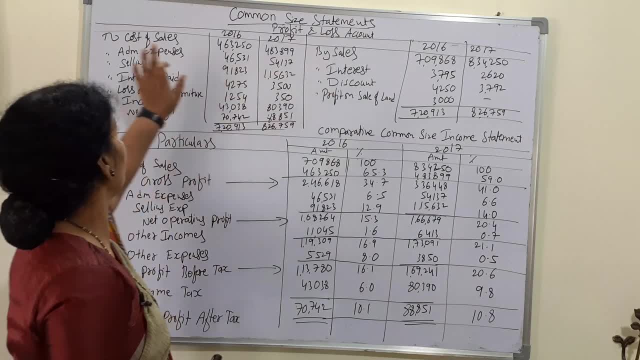 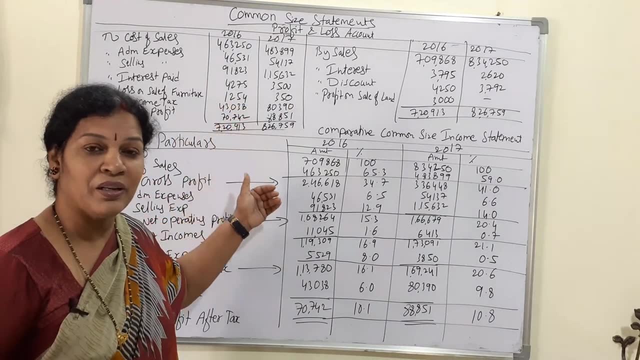 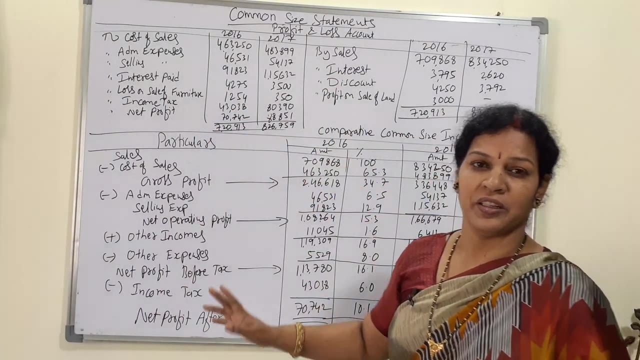 Now what is given to us Sales? Sales minus cost of sales will get gross profit. Gross profit minus administrative expenses, Administrative expenses will get net profit, But before tax, like that. So I have done already the problem. Easy to explain And it will take lot of time for me to take the calculator and working out. 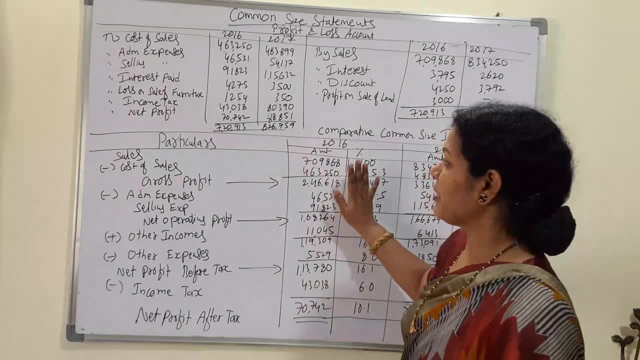 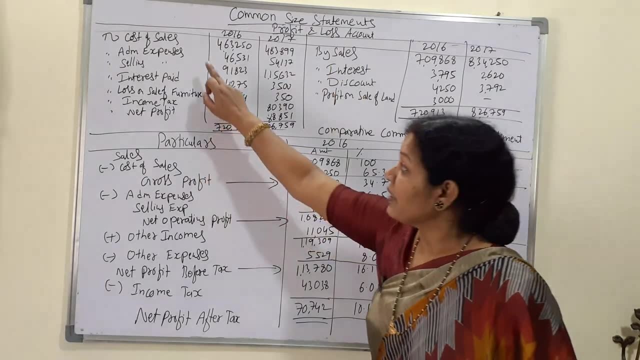 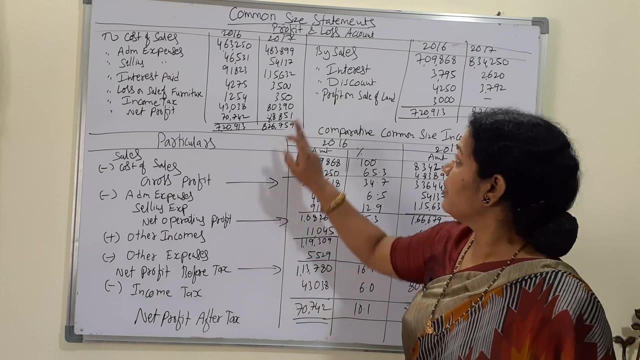 So easy way is that you can save your time also. Now let me explain this comparative common size statement. First, we have taken sales. This is sales Sales minus cost of sales, Sales minus cost of sales. you are getting gross profit After getting gross profit. next, administrative expenses and selling expenses. 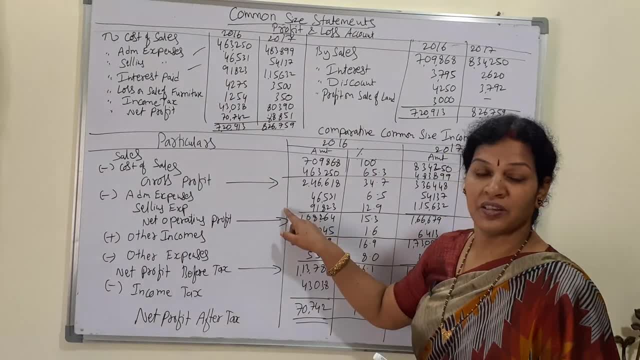 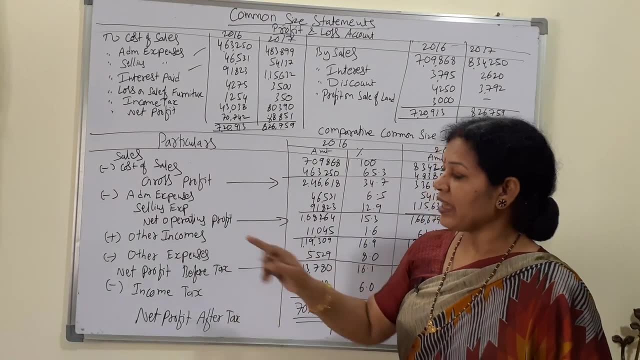 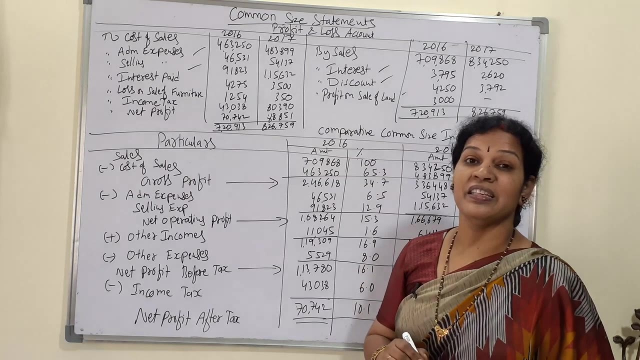 Administrative selling expenses deducted. After deducting, we are getting net operating profit. Net operating profit From that- other incomes. What are the other incomes here? Interest discount, profit on sale of asset, These are the other incomes. All these incomes, we are adding it. 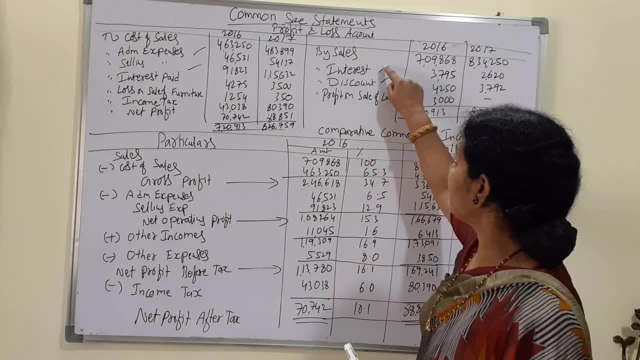 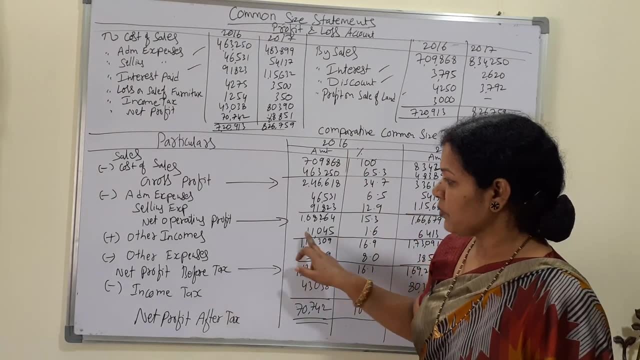 Do you know the profit now? So we are adding other incomes. These three together Interest discount profit on sales. So these three added we are getting 11,045.. So then after that add other expenses. Sorry, minus other expenses. 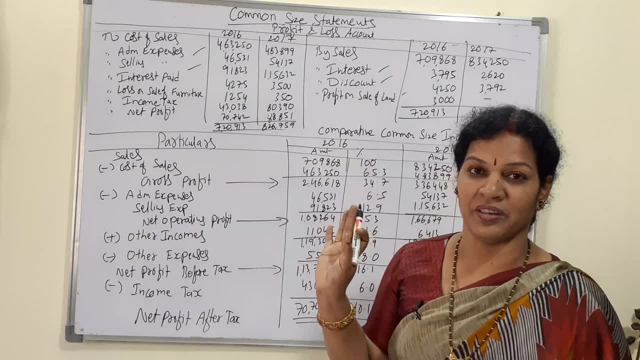 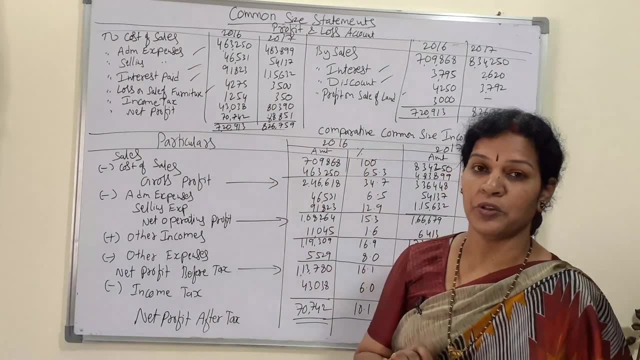 What are the other expenses? Administrative selling already we have taken. Other expenses means here Interest paid loss on sale of furniture. These two are other expenses, Only two: Interest paid loss on sale of furniture. If you add these two that we are taking it. 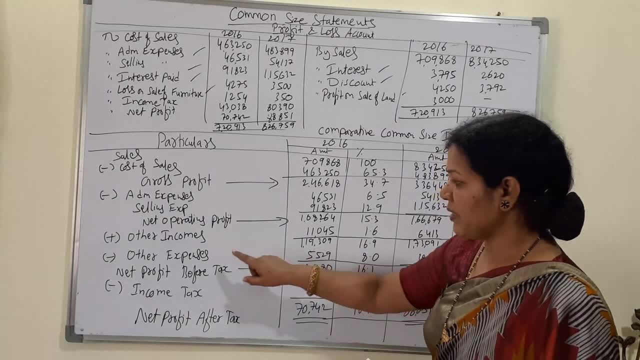 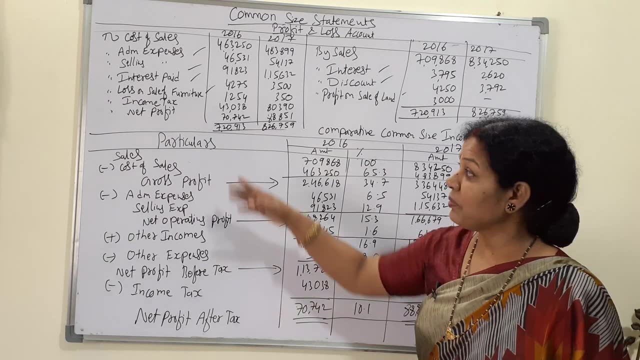 As other expenses, Other expenses we have deducted. So this is net profit before tax. Why we are saying: before tax There is a tax, is given income tax. If income tax is not given, Then we would have taken it as a final net profit. 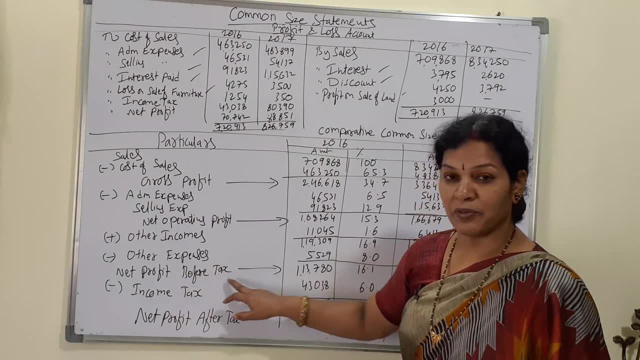 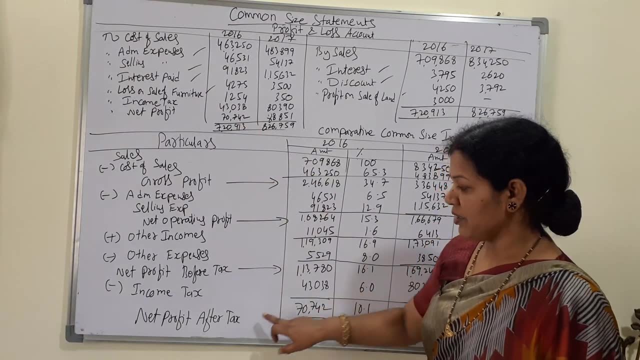 Income tax is there. That is why we are saying net profit before tax. Now what to do? Deduct income tax, Income tax 43,000.. So that deducted, So you are getting net profit after tax. So this is general pro forma. 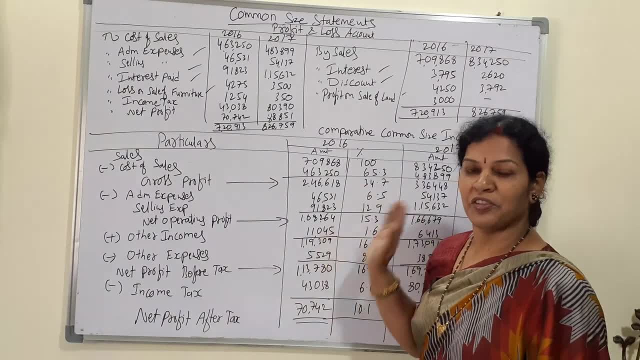 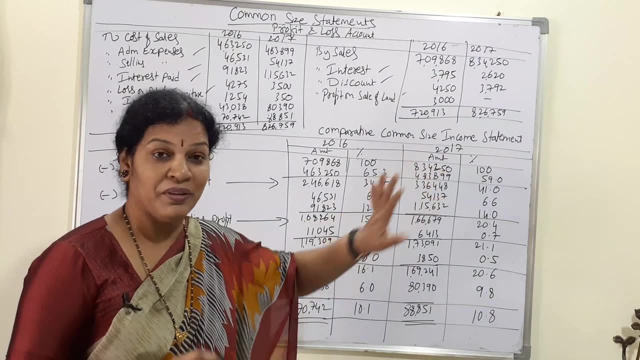 This pro forma. remember Now calculation. anyway, it will be easy. Now, coming to the calculations, We have two years: 2016 and 17.. We are not seeing increasing or decreasing, We will see only the same year. Percentages will calculate. 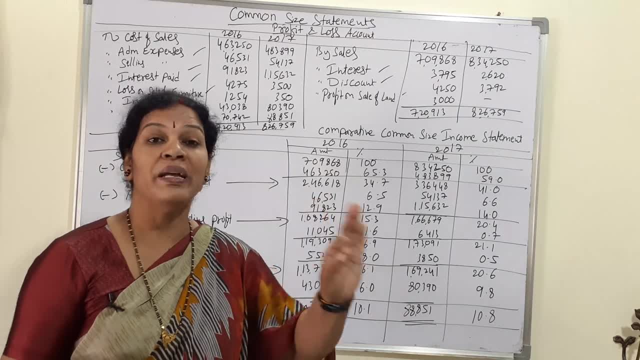 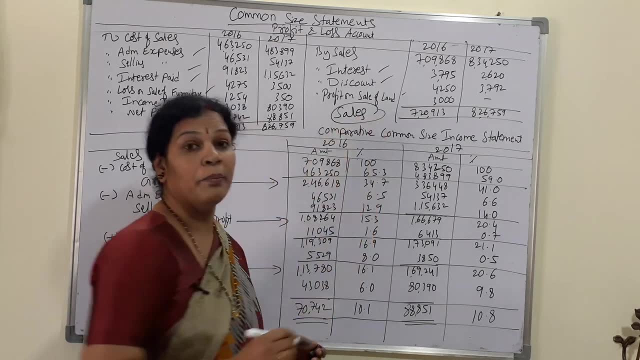 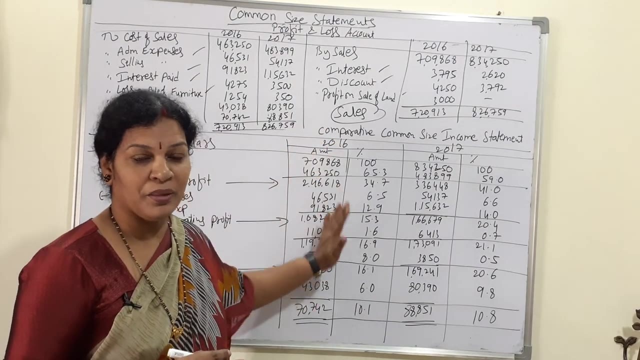 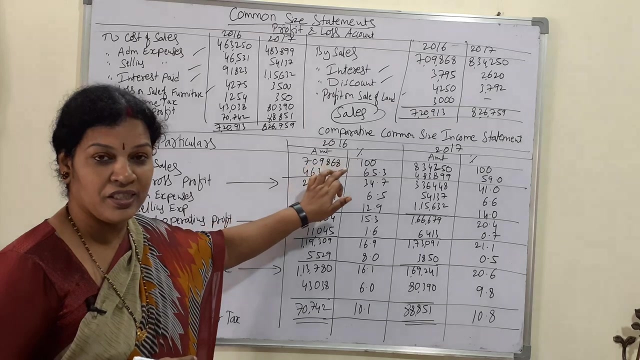 How do we calculate that? As I told you, Basis here, sales, Basis here. always remember, Sales is the base Based on sales will be calculating all the percentages. Say, suppose, sales for the 2016 year is 7,09,868.. 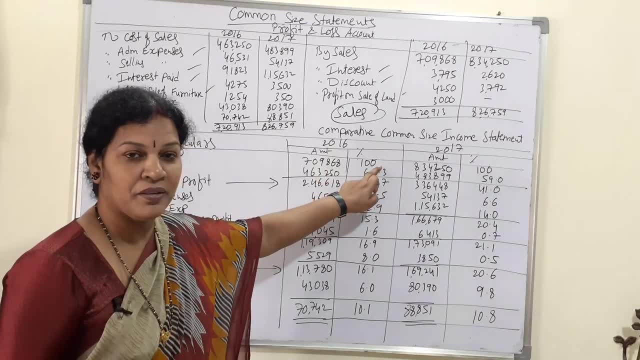 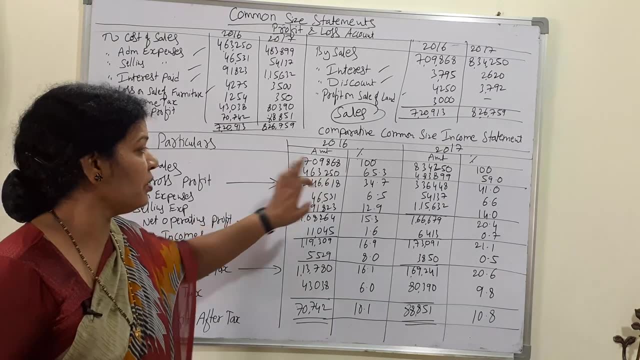 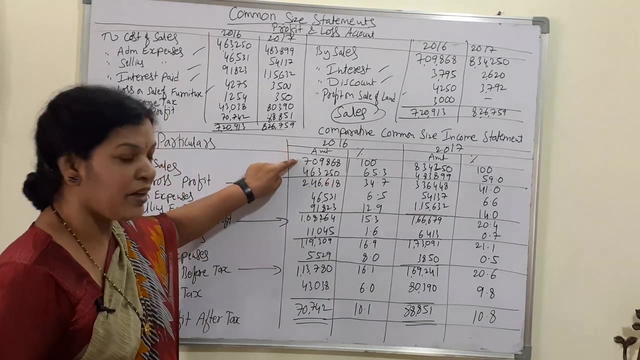 This is base now, So we are saying it as a 100.. Next one is that Cost of sales. Cost of sales are 4,63,000.. To know the percentage, how do we calculate 4,63,250 divided by 7,09,868 into 100.? 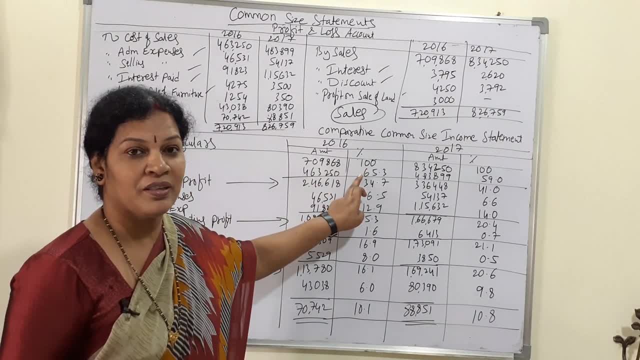 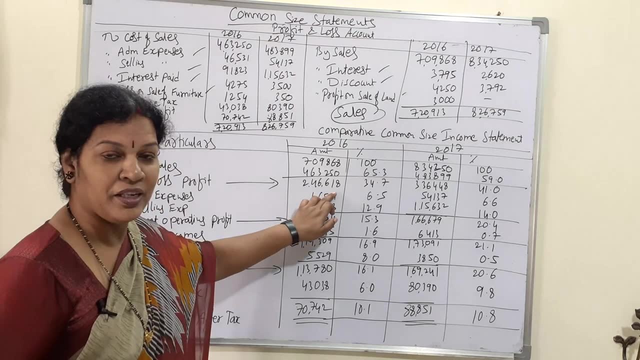 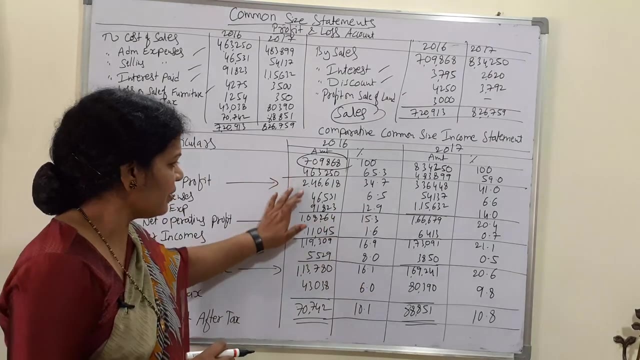 So that we get 65.3%. In the same way, Gross profit, we got Gross profit percentage. how do we get 2,46,618 divided by this? This is common. Whatever you are calculating This amount divided by sales. 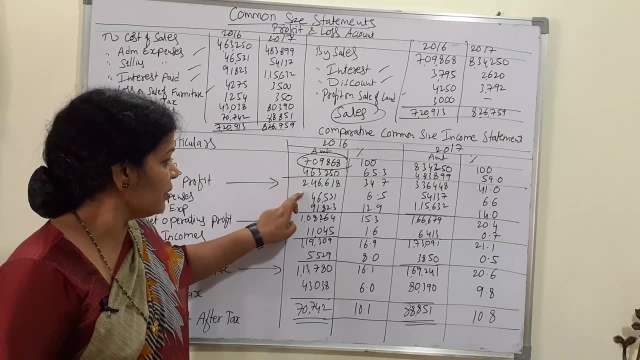 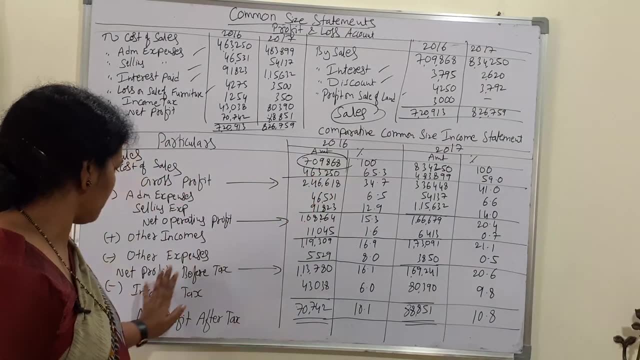 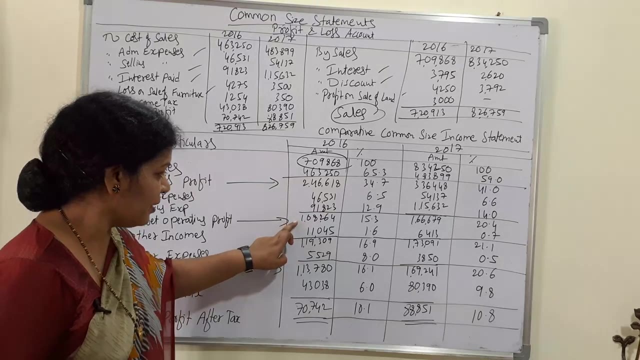 Because sales is the base. So this gross profit divided by sales into 100, you got for 34.7.. In the same way, any amount. Suppose say we are taking net profit, Net operating profit, This percentage you want to calculate This amount net operating profit. 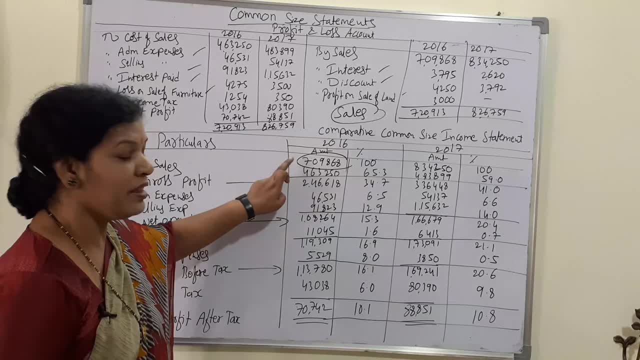 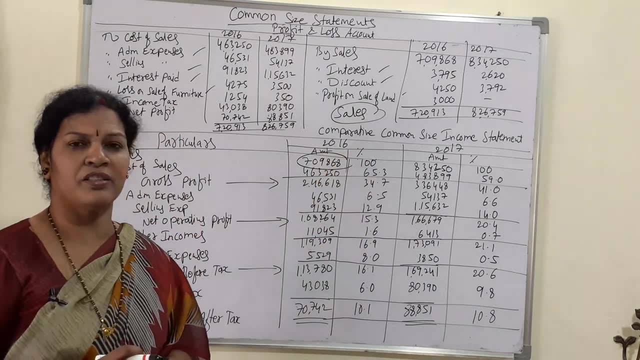 Amount, that is 1,08,264 divided by sales into 100.. So that you get 15.3.. Like everything, we have calculated Simple one, So are you getting it? Calculate any amount, That amount divided by sales into 100. 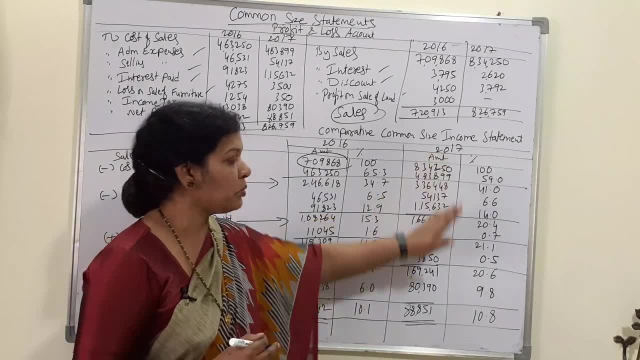 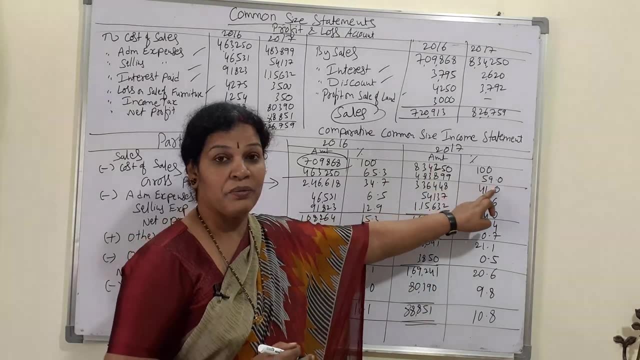 So this is 2006 year. In the same way, 2007 year, 2007 year also. as per the proforma, we have written everything For calculation. sales is the base, So we have written sales as 100.. And any amount we want to calculate. 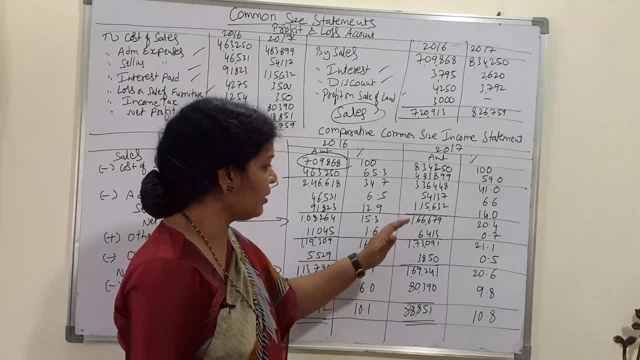 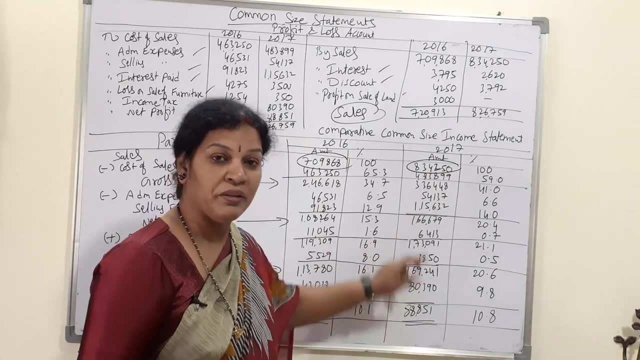 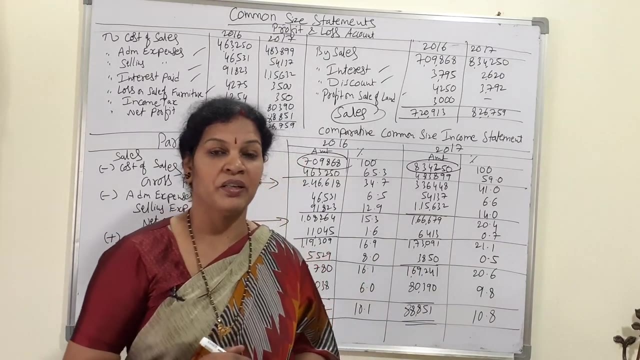 Any of this percentage. you want to calculate This amount divided by sales, This amount, any amount divided by sales into 100. So that you get the percentage. So like you can calculate the common size income statement. Remember one thing is that In common size income statement, 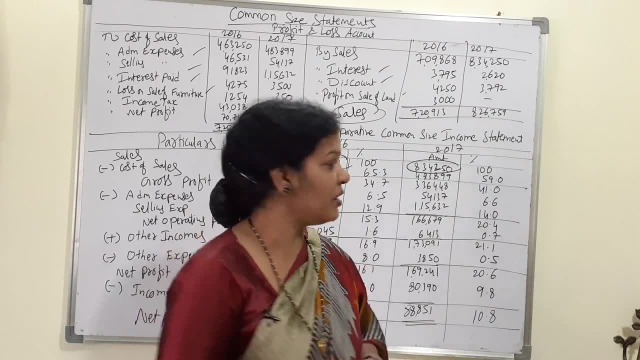 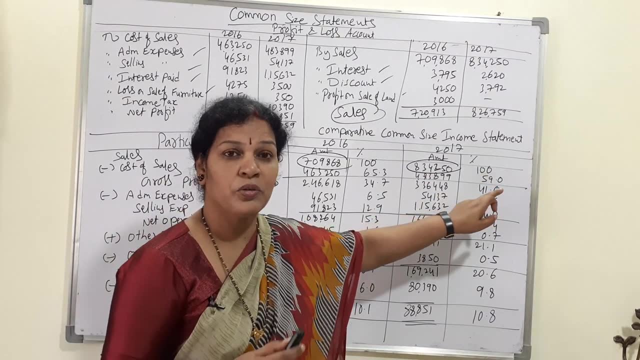 Mainly, we are giving weightage to the sales As per the sales. When sales are 100%, What is this cost of sales As per the sales? it is 59%. So it will be easy for us to understand When sales are this much. 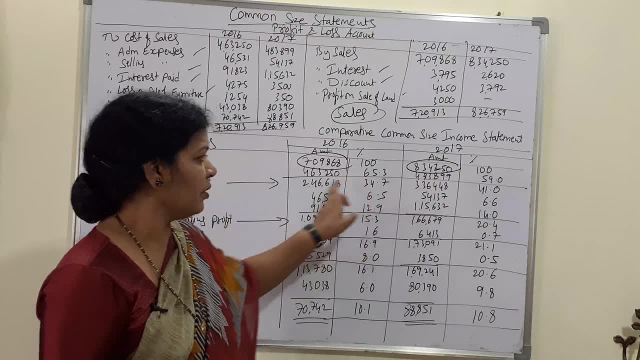 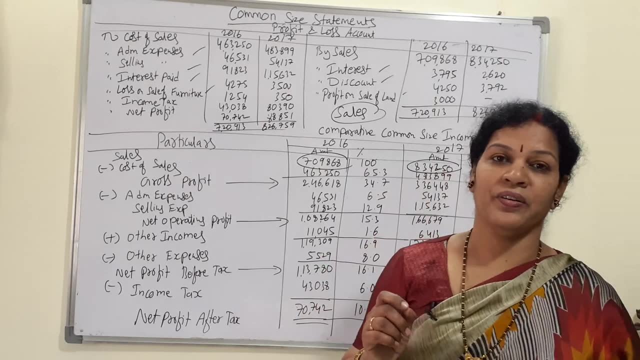 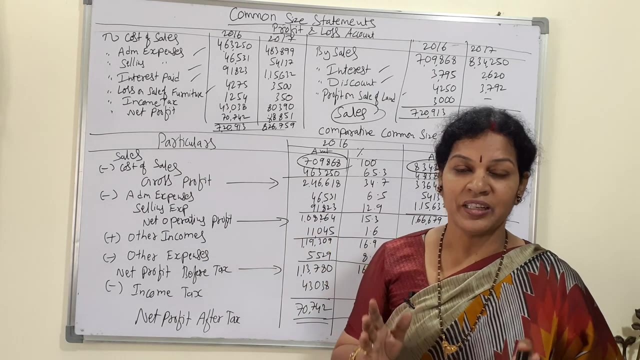 What is the GP? Gross profit? is this one? What is this GP? GP is 41% compared to sales. So this will give you a clarity of sales And any item, any transaction. So this we call it as a common size income statement. 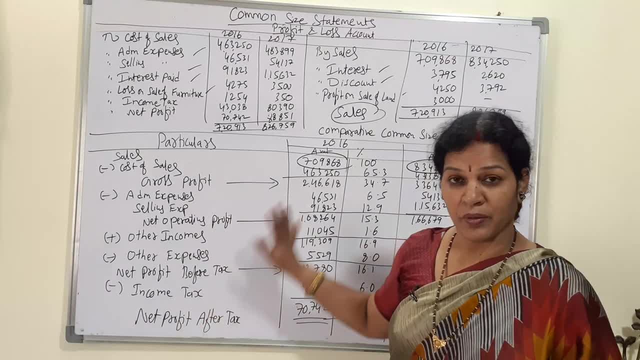 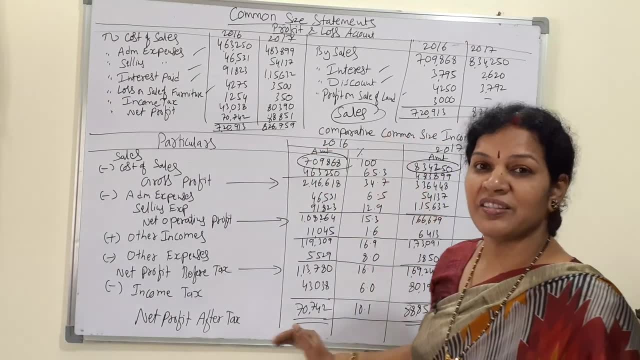 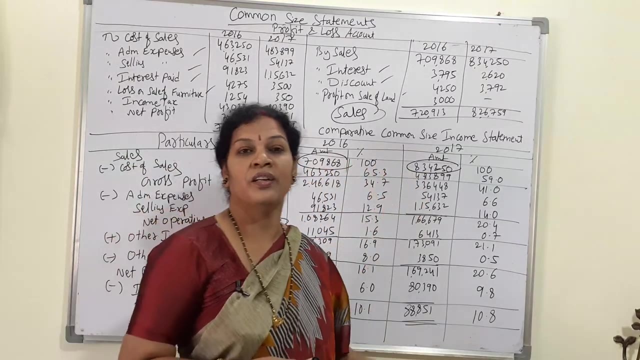 Proforma is same like previous one, Only the calculations we are taking, Rather than comparing from 2016 to 2017.. We are taking same year, only Same year calculations, Taking base as sales. That's it. This is And coming classes. 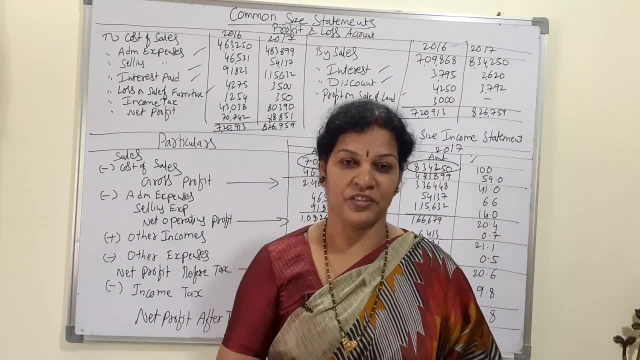 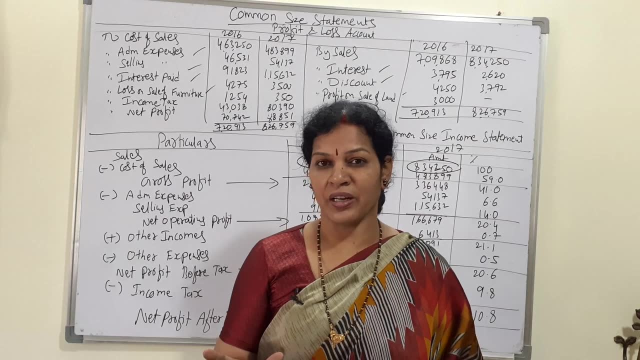 We will work out some common size balance sheet. In common size balance sheet We are going to take base as The total current assets or total current liabilities. Both will be same: Assets and liabilities. The same one we are going to take. 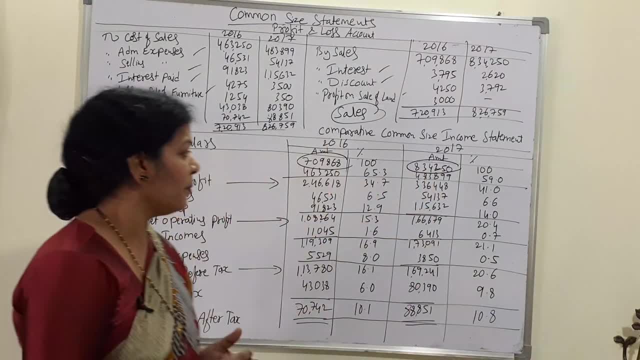 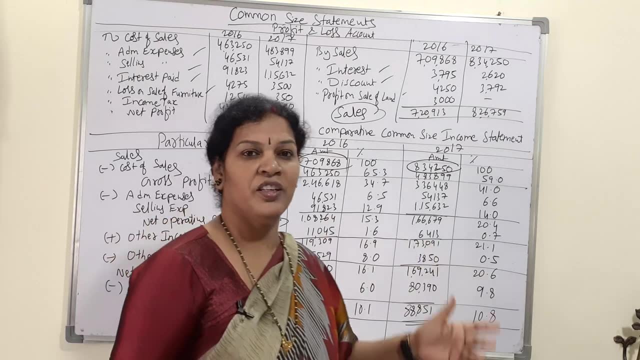 So hope it is useful. Please watch, Please pause the video And note down this problem And it will be easy for you to understand Common size. If it is given in the exam Easily, you can score. So please go for your test book. 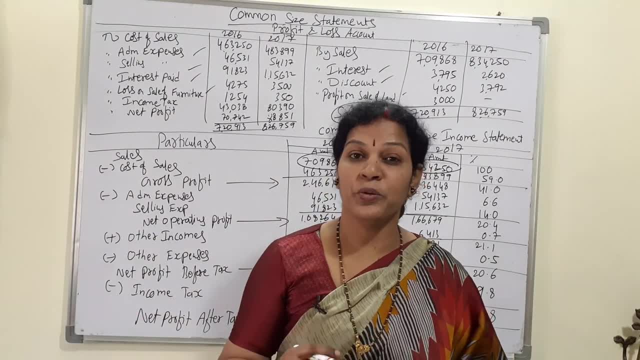 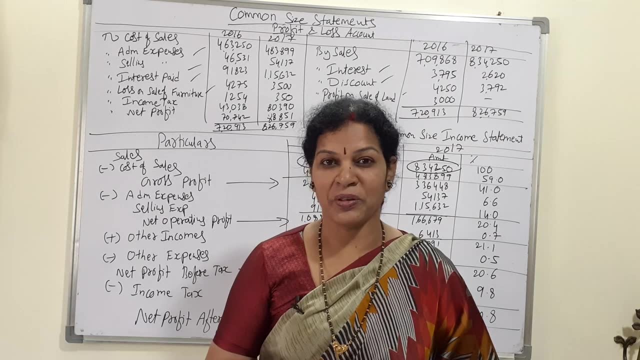 After work outing this problem, Take out your test book And try to work out more problems So that you will have confidence. Practice makes you perfect. So thank you very much for your feedback. Please stay in touch with lot more subjects, Lot more topics.